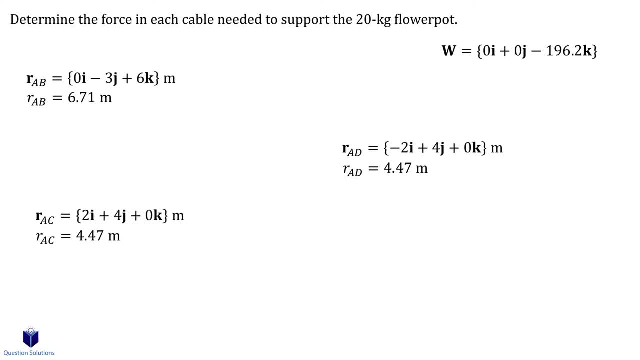 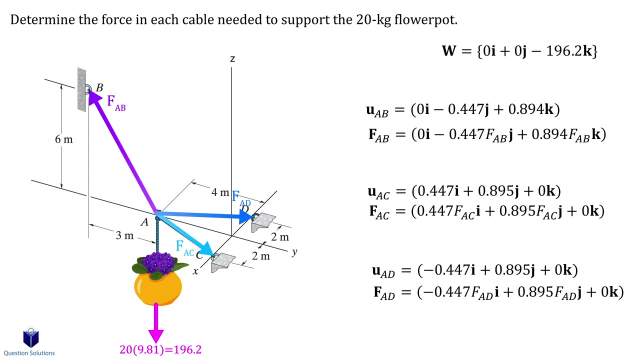 Now comes the unit vectors. So we're just dividing each component of our position vector by the magnitude. We can finally express each force in Cartesian form. All we do is multiply the magnitude of the force by the unit vector. Now that we have all the forces, we can equate. 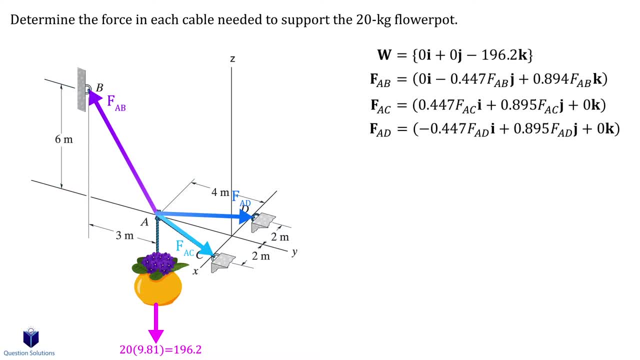 all the individual components to zero. Now we can calculate the magnitude of the force in Cartesian form. Let's start with the x components. So we see that we have two x components. Both of them added together must equal zero. Next the y component. Lastly, we have the z components. 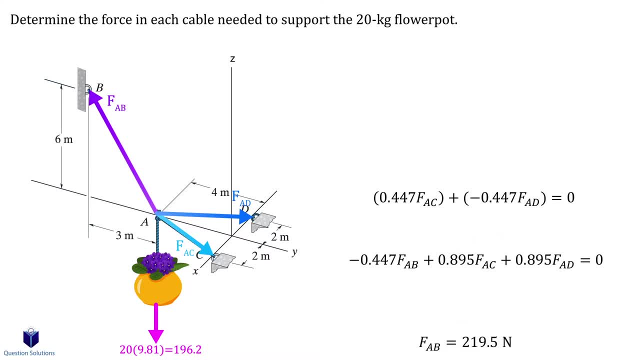 From this equation we can directly solve for force A- B. Now we have two equations left with two unknowns. Let's solve them. Don't forget to use the value of force A- B we just found. Those are our answers. 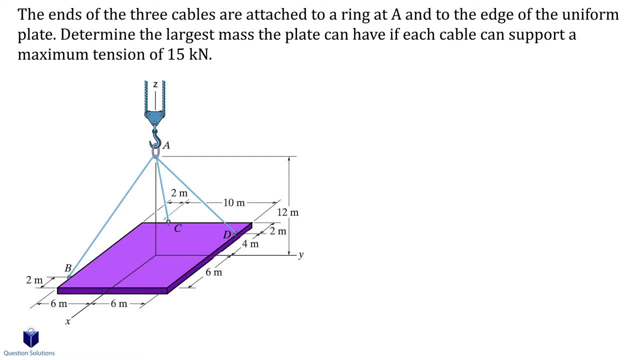 a look at this problem where a plate is hung from cables. Each cable can support a maximum tension of 15 kN and we need to find the largest mass of the plate that can be hung. So first we need to express the forces in each cable in Cartesian form. The process is identical. 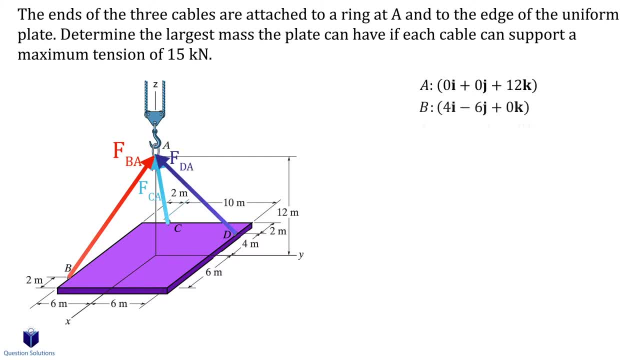 to what we did before. Let's start with our locations. Now that we have our locations, let's write our position vectors for each cable. I am assuming all the forces start from the plate and travel towards point A, so the position vectors will be from B to. 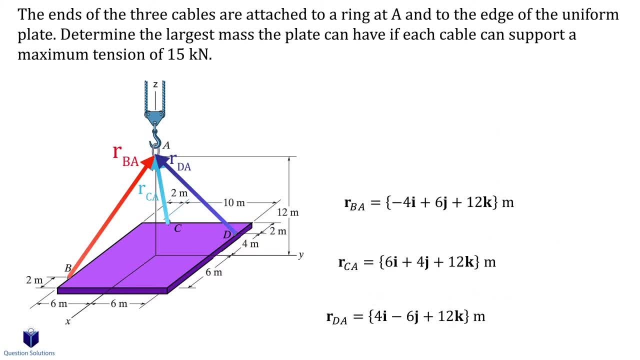 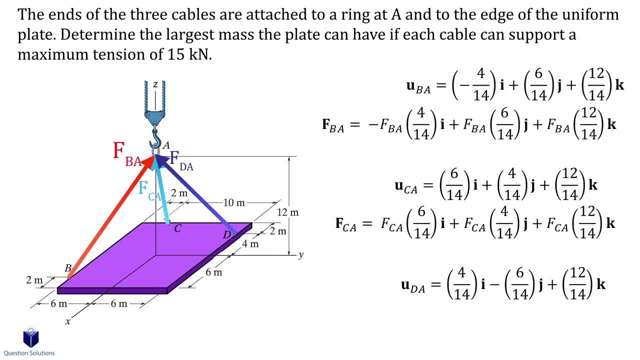 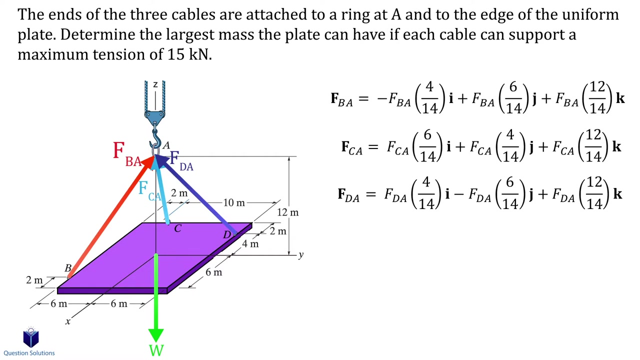 A, C to A and D to A. Now that we have the position vectors, it's time for the magnitudes. Next is the unit vectors. Now, to express each force, all we need to do is multiply the magnitude of the force by the unit vector. Don't forget: we also have the weight of the 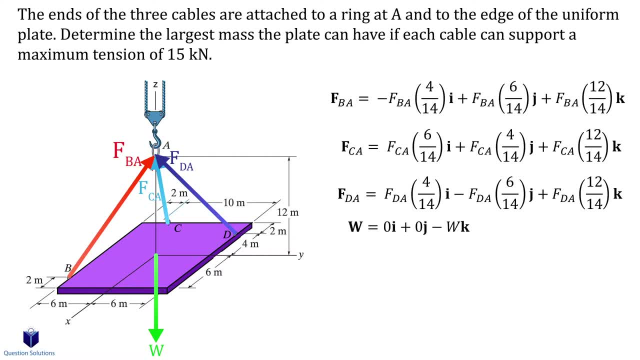 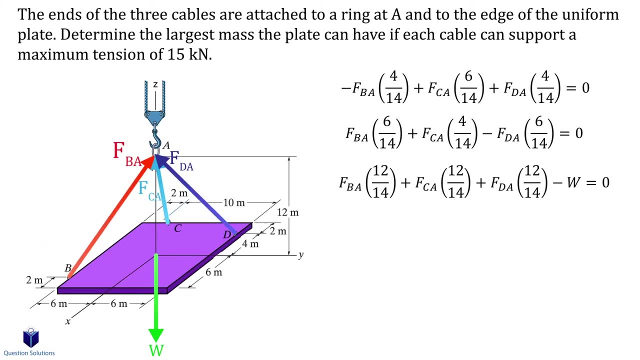 plate which will be straight down. Now we're going to equal each component to 0.. First the X components, next Y components. lastly we have the Z components. Now we need to make an assumption. Let's say we assume cable AB will carry the largest force possible. So 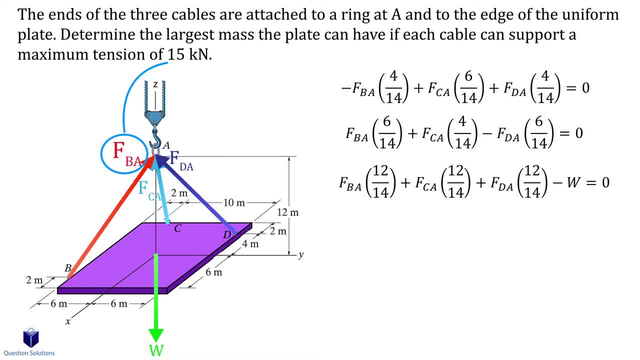 we will assume it to have a tension of 15kN. that's the max a cable can support. If we do that, we need to check to see if the other cables are less than or equal to 15kN. If they go over, then cable AB can't be 15kN. 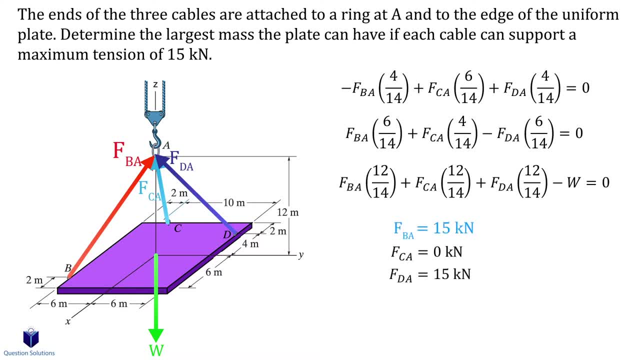 Let's assume cable AB is 15kN and solve the equations. We get the following values: This tells us that cable CA carries no force and cable DA also carries the maximum it can, So all the conditions we require are met. Now all that's left is to divide the weight. 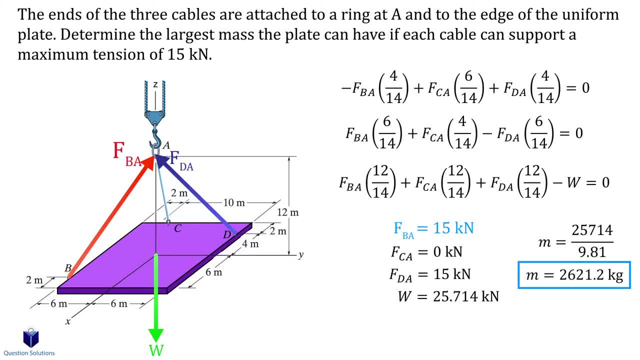 by the acceleration. But let's say we assumed cable CA to be 15kN, Then when you solve them you will see that no solutions exist. If we assumed cable DA to be 15kN, then we will get the following: 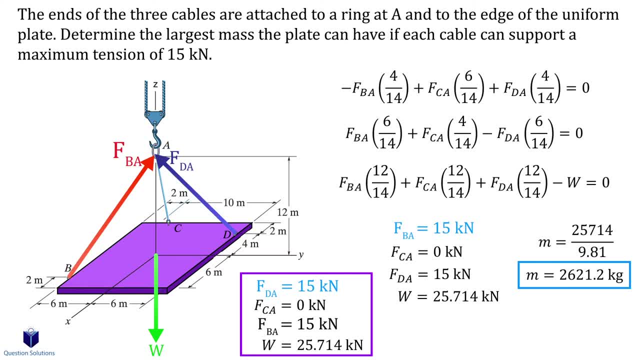 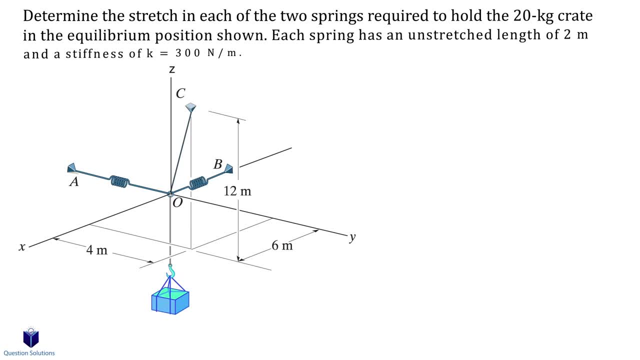 answers. So the same answer as when we assumed cable BA to be 15kN. Let's take a look at one last example involving springs. In this question, we need to find the stretch of the two springs in order to hold the 20kg crate in equilibrium. So the way to solve it is pretty much the. 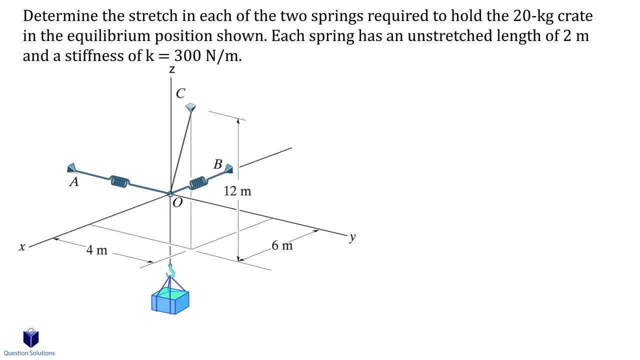 same as before, where we need to express each force in Cartesian form. If we look at the two springs, spring OA lies on the negative y-axis and spring OB lies in the negative x-axis. That means spring OA will only have a j-component, while spring OB will have an. 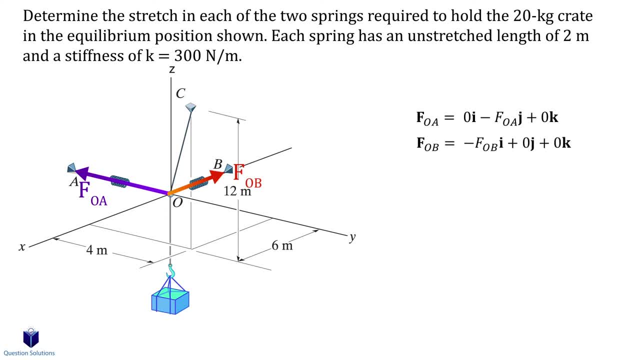 i-component. Next, we need to express the force in cable OC. So the position vector for OC can be written like this: Now the magnitude, The unit vector, comes next. Finally, we can express the force in Cartesian form. We have one more force, which is the weight. 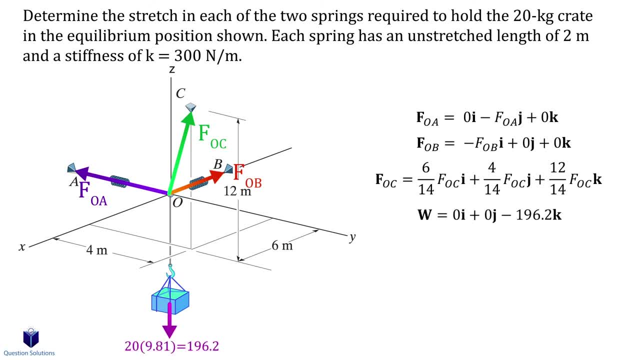 of the crate. That can be expressed in Cartesian form like this: since it's straight down and only has a k-component, Now we can equal each component to zero. We now have three equations with three unknowns, So let's solve them. To figure out the stretch in each of the springs, all we need to do is: